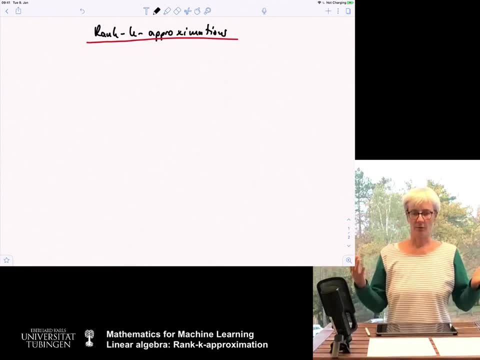 rank of a matrix. So if you have a matrix of rank one, once we know all columns, once we know one column, essentially we know all the other columns. they're just multiples. If we have a matrix which has a low rank, k, once we know k columns, we know all the other columns. they're just multiples. 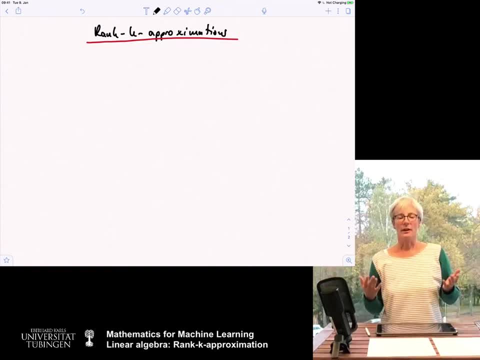 We essentially know the rest of the matrix. And now the idea is that in many cases you want to approximate a big matrix by such a rank k matrix to reduce the complexity of the problem. And here is now the solution that you can, or the simplest solution that you can, do for these. 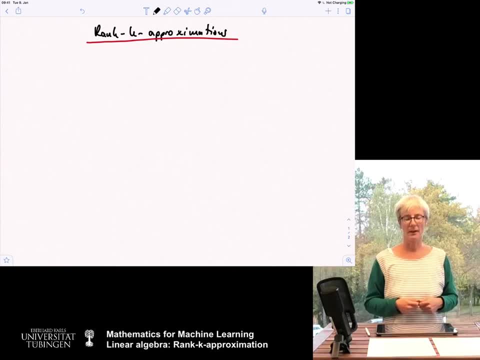 kind of problems in terms of the singular value decomposition. Now, before we can actually define what I mean or express the theorems that I want to tell you, is we first of all need to say in which sense are we going to approximate a matrix, So in which sense are two matrices close to each other? 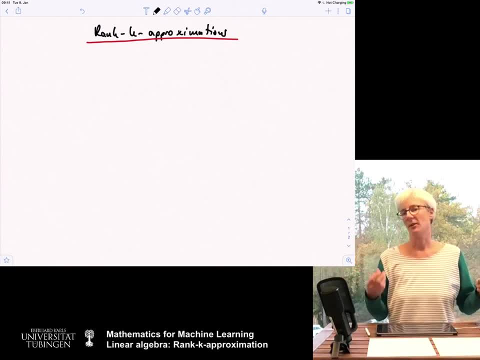 And you can guess that what we need to express it is we would either need a metric on the space of all matrices, or maybe a norm. And now the first thing that we're going to look at are matrix norms, and I'm going to show you what are the most popular matrix norms, and then we are. 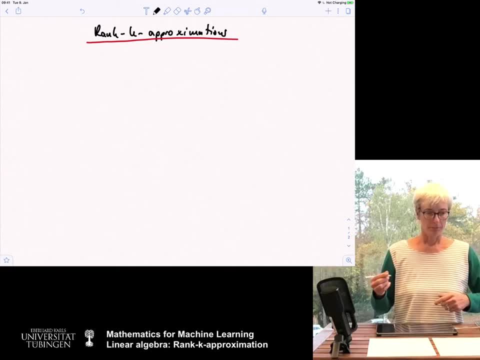 going to see how we can discuss them, So maybe this headline is not entirely appropriate. I might want to delete it for now and maybe write matrix norms first. Matrix norms. Okay, so we're given a matrix A and in general it's not necessarily in a square matrix, it can also be a rectangular matrix. 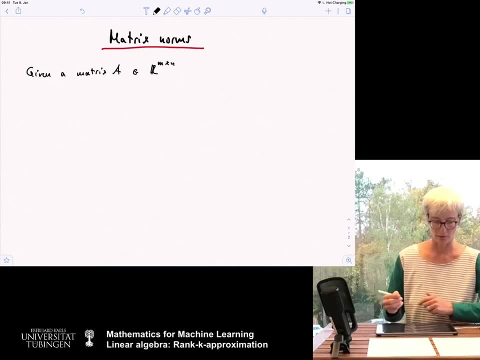 For some of the norms it's better if it's squared, but let's try to see it like this and define the following norms. So the first and now. I'm simply giving you a summary of what are some of the norms that occur very often. 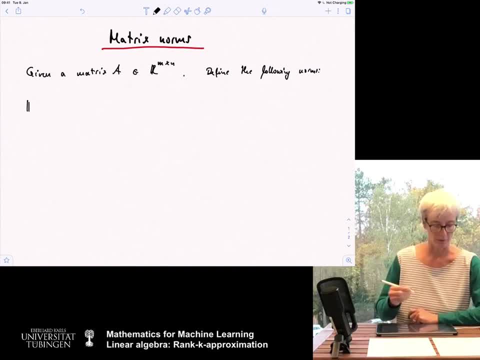 There are millions of matrix norms. We just consider the most important ones here. So what is often called the maximum norm of a matrix, and sometimes people write a max and sometimes people write infinity- This is just the maximum entry. You look at all, the maximum of all i's, j's a, i, j. 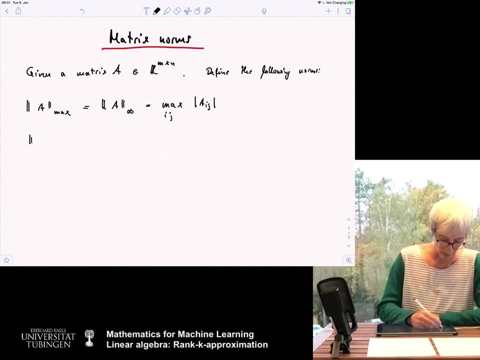 This is sort of a very simple norm. Then what else do we have? We have what is sometimes called the one norm. And then what else do we have? We have what is sometimes called the one norm, which is just the the sum over all ij's of the entries of this matrix and absolute values. 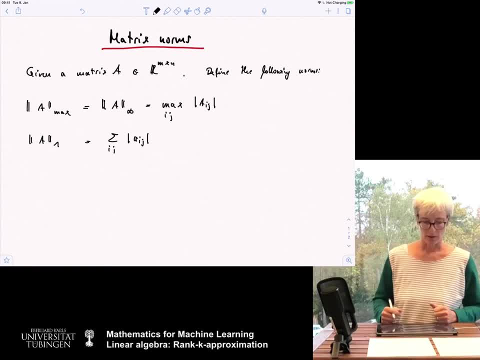 This is something like a one norm of a vector just applied to a matrix. Maybe the first one is something like the infinity norm of a vector just applied to the matrix entries. and I see I made a mistake here. I should have had lower case a's here. 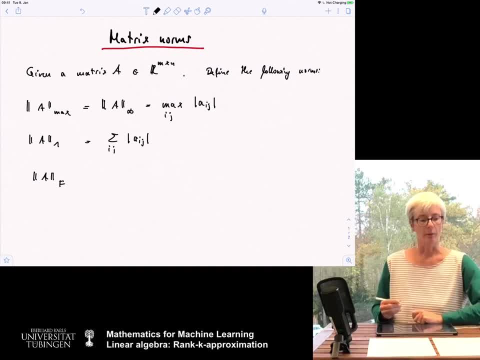 And then there is what is called the Frobenius norm, And this is essentially if you apply the two norm to the entries of the matrix considered as a vector. So you sum over all ij's a ij square and take the square root in the end. 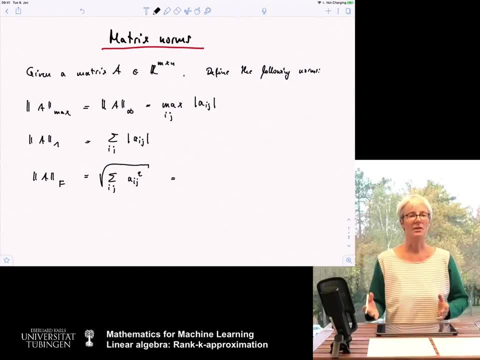 And there are a number of equivalent expressions and it is not completely obvious, maybe, that these are equivalent. So each of these equality signs that I'm going to show you, I'm going to show you state now, in fact, would require a proof, but I don't want to give it because we simply 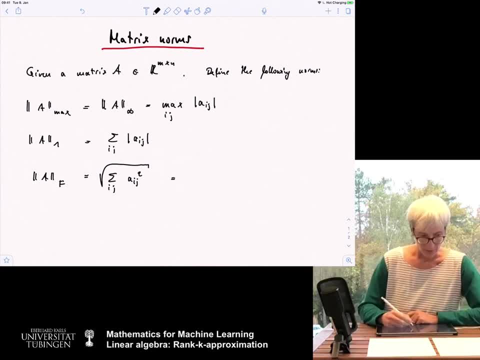 don't have the time, but you can read that up. This is in fact the same as if you take the square root of the trace of a transpose a, And this is also essentially if you take the sum of the singular values. sigma i: squared where. 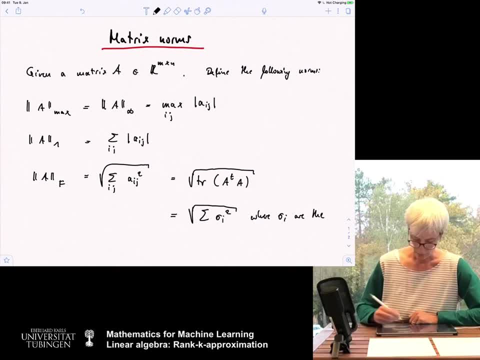 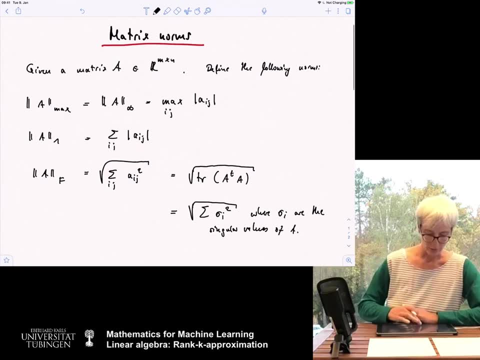 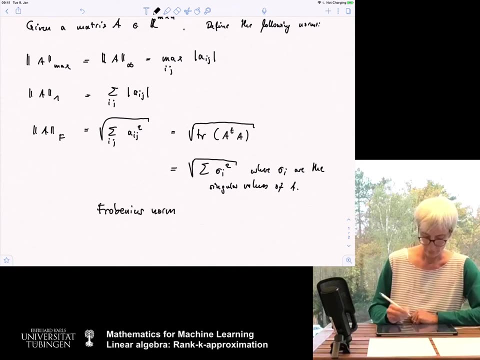 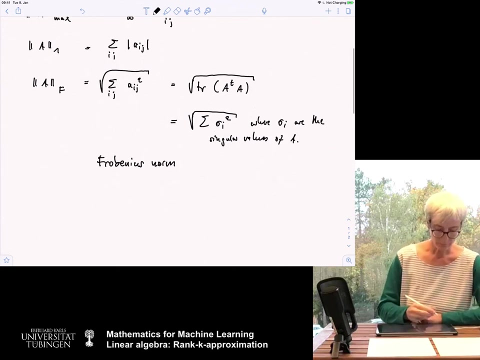 sigma i's are the singular values of a, And this norm is called the Frobenius norm. And then there is yet another norm that is important, which is the operator norm, Which is defined as follows: Sometimes people write as a2,, sometimes they don't make any index, and now this is either. 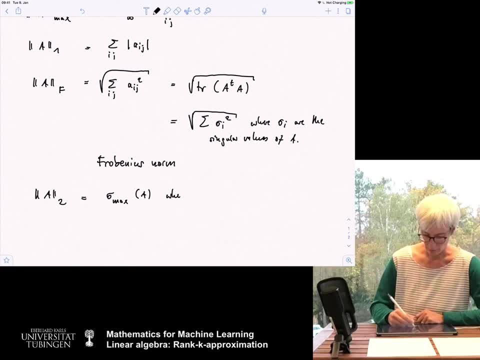 sigma max of a, where sigma max is the largest singular value And you can also write it in. if you already know what an operator norm is, I'm going to explain it a bit later. Um, You can also write this as the maximum overall vectors which are non-zero of a x norm of: 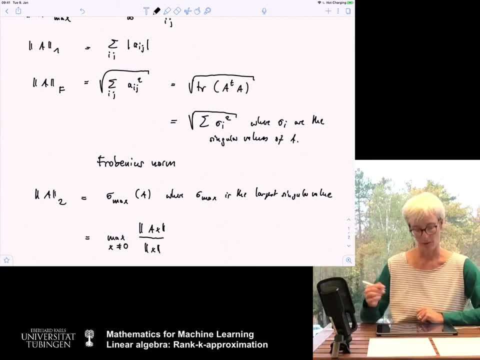 a, x divided by x. And now the question is: what is the norm I'm currently talking about? So these are the Euclidean norms, The Euclidean norm on vectors, On vectors in Rx. Okay, Okay, Okay, Okay. So the Euclidean norm is the maximum of the norm that you can define as a two norm matrix. 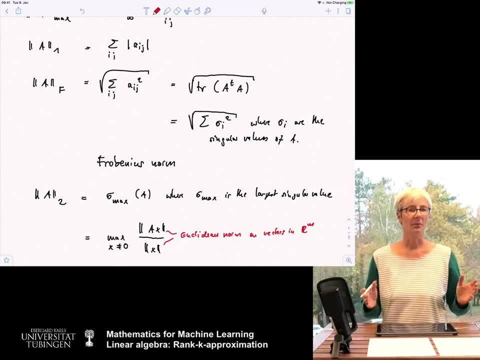 And then the norm on the matrix is actually the norm on the matrix. So in the matrix you can define it as a two norm or m. Yeah, And I want to give you one caveat. The business of matrix norms, this is really, it's a bit of a disaster, because the notation 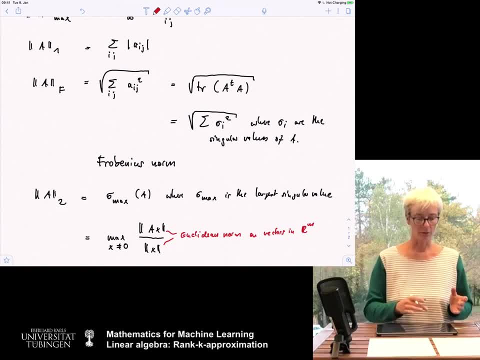 is really different in different books. So there might be people who use the two norm notation to denote the Frobenius norm, because it looks like taking the square norm of something, And even for the maximum or infinity norm. so there are millions of different ways in. 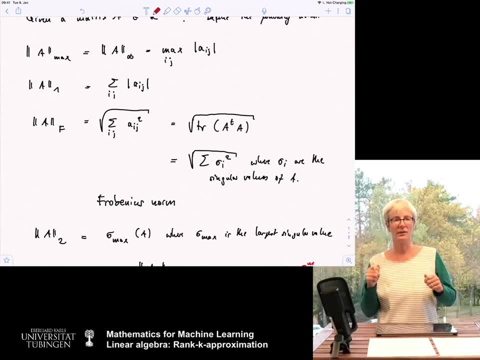 which people can define the norms and they add all little kind of indices, ones and infinities and twos, And there are many, many different versions. So whenever you read a paper or a book and it says something about a matrix norm, you first need to check what this norm. 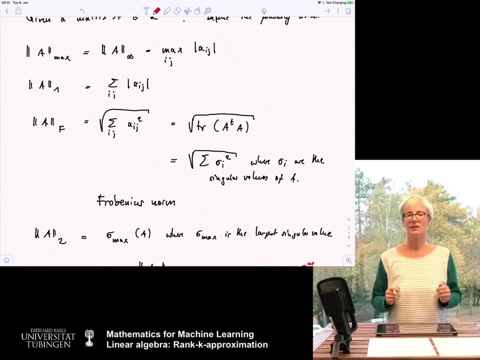 is, The notation is completely non-unique and it can be a disaster, but there's no way around that, And I even got confused when I prepared this lecture and had to read up all of it again. Here is now one notation. I'm not even sure whether we are going to. 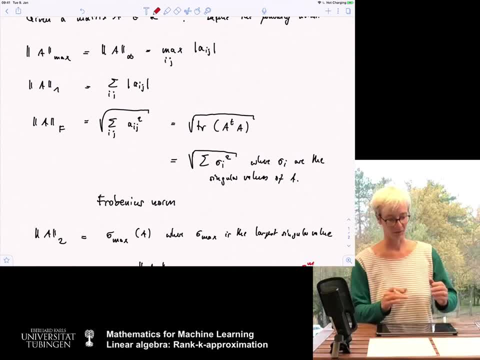 use it consistently in the rest of the lecture, but for this lecture we're going to stick to this notation. I think the two norms that are most important for many applications in machine learning are the Frobenius norm and the two norm, the operator norm. Maybe I write. 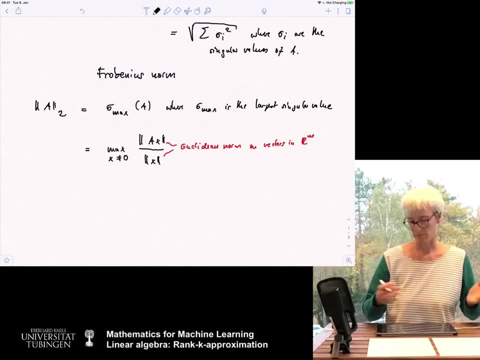 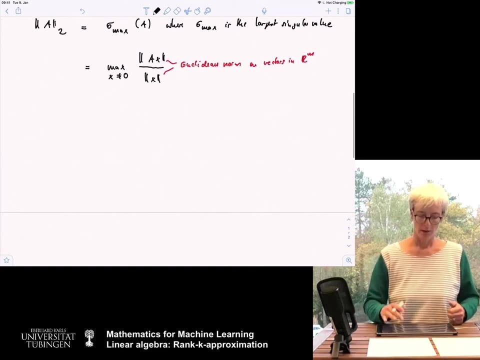 here as well, I don't need to write it. Okay, And now we have these norms, and now I want to define what is a rank k approximation and then want to state that these rank k approximations of matrices are optimal in some of these norms. So now comes the next heading: rank k approximation. 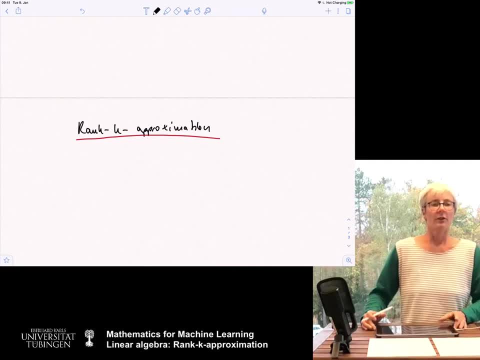 So essentially a matrix. if a matrix has full rank, say, and we approximate it by a matrix of rank k, then this is a rank k approximation. But of course we are not interested in any odd rank k approximation. but we want to have a good approximation And here is how we define. 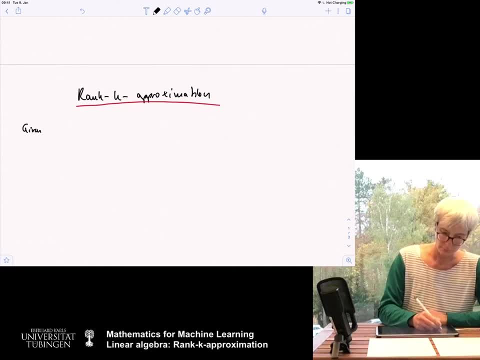 that, Given a matrix A and its singular value, decomposition, we have a matrix A and its decomposition, u sigma v transpose, And now we define a matrix A k And we are given also k, a natural number. We define A k in the following way: 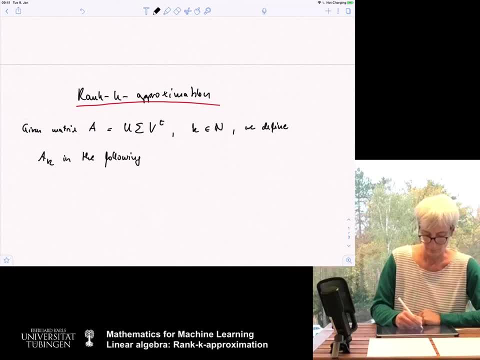 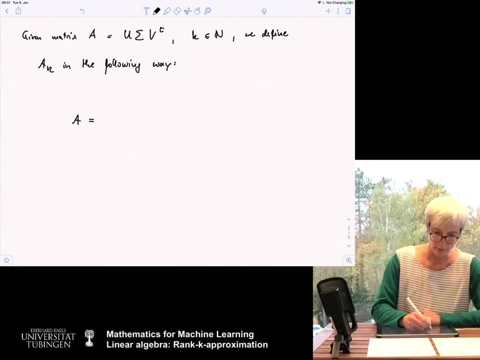 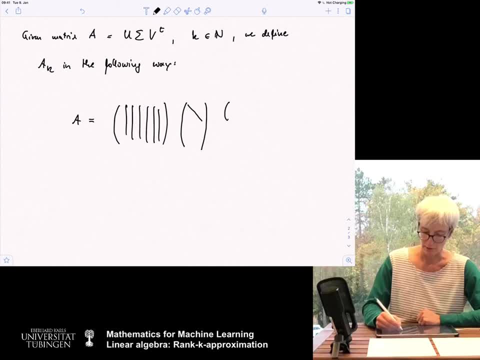 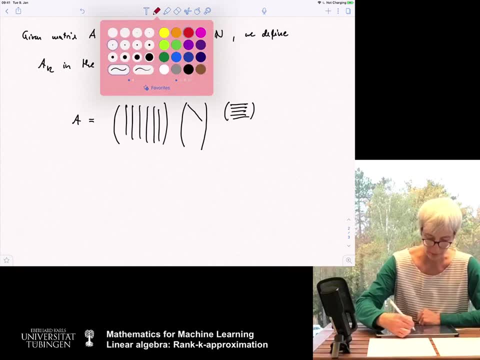 this diagonal matrix consisting on a diagなl and zero everywhere else, And then we have that small matrix consisting of lots of rows. Now the rank k approximation thanks to first k columns here. So here we take, say, the number of rows that we write, but we also 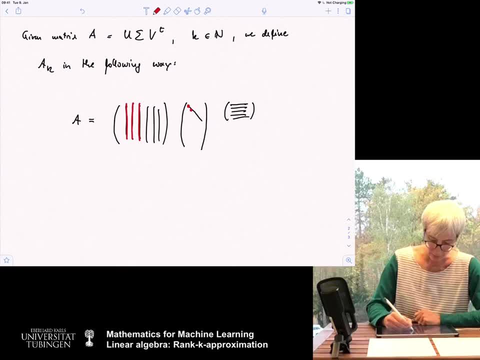 first three columns. here we take the first three entries, and here we take the first three rows and the rest we simply set to zero. so, um, i just write take, oops, it's two, so we take the first. take first k columns of u, the first k entries of sigma, and of course here i assume that the entries of sigma are. 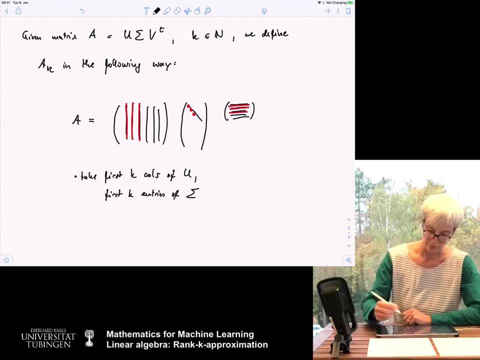 sorted in decreasing order. maybe i should define this here, maybe i write it here- where the entries in sigma are sorted in decreasing order. so the most important ones are the largest one and they come first. so we take the first k columns of u, the first k entries of sigma and the first k rows. 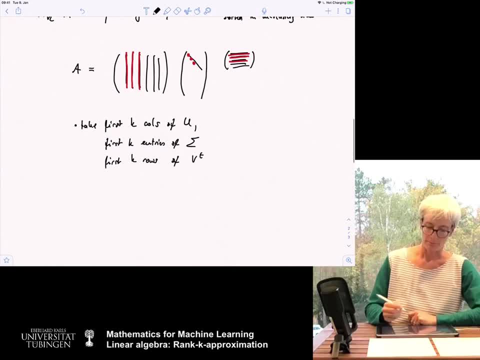 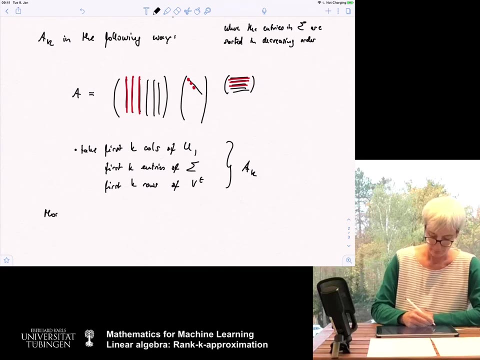 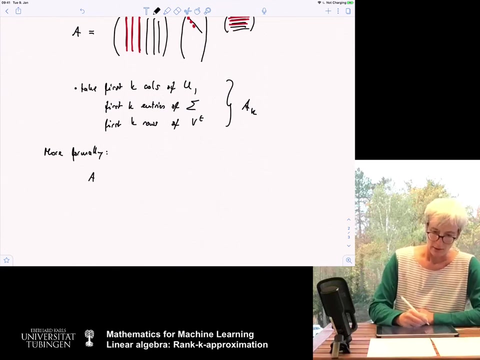 of v, transpose um, and then we compute the product and this gives us a k. okay, if you want to have a formula, you can also write this um more formally. we can. we can write a k as the sum over i equals one to k sigma i, u, i, v, i transpose. 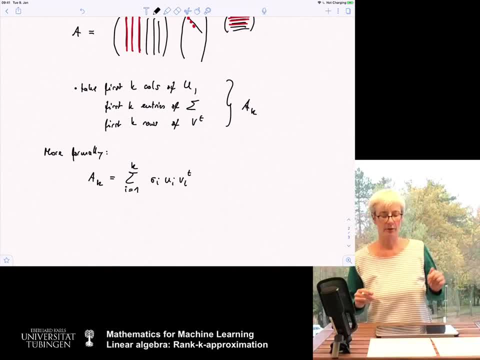 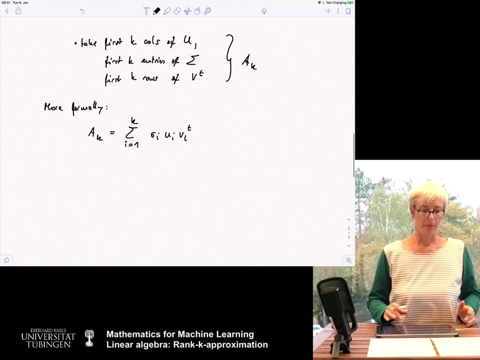 okay, so we just take the first k eigenvalues and the corresponding left and right eigenvectors. okay, and now? um, you can guess already where we're heading to. probably this matrix ak is a good approximation of the matrix a in a certain sense, and indeed this is the case, and i want to give you 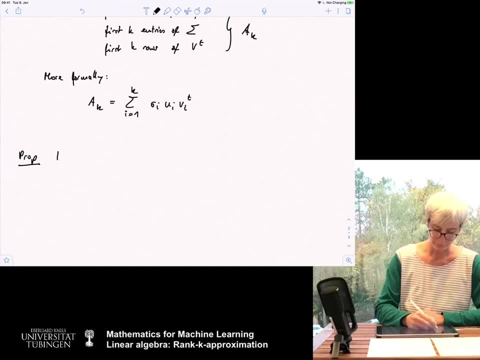 two propositions. proposition the first one is: let b be any rank k matrix in our m times n, so the same size as the matrix a. then what we have is: if you look at the frobenius norm difference between a and a k- let me first write it down- it is always lower or equal than the frobenius norm difference between a and b. 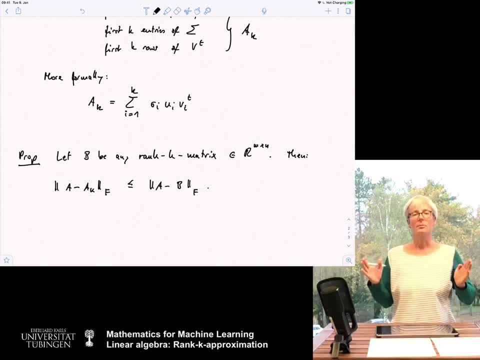 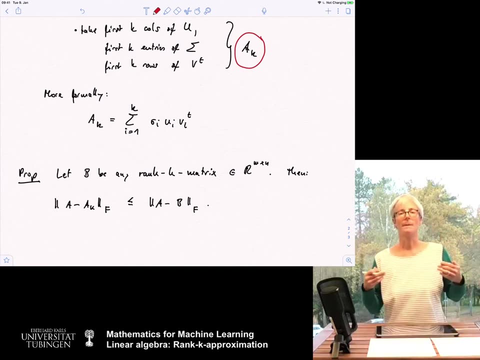 so this means intuitively, no matter which matrix b we are going to plug in, in terms of the frobenius norm, we can only get better if you use a k, and a k is the matrix that we just defined here. maybe i make a little circle around it. so this is sort of, if you take the first. 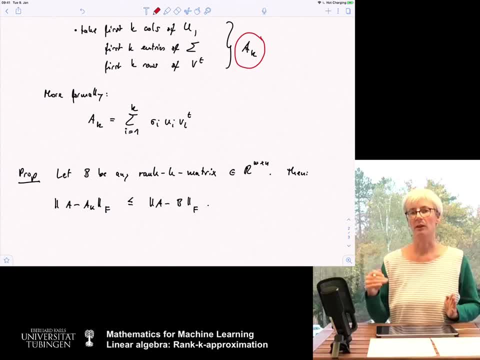 k singular values and you and the corresponding singular vectors and you set the remaining stuff to zero, then this is the best thing that you can do. if you want to approximate your original matrix by a rank k matrix and you measure the distance in terms of the frobenius. 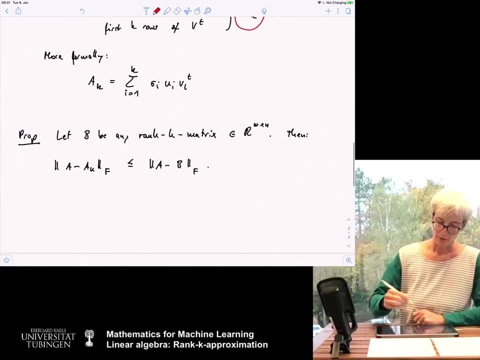 norm. so maybe intuitively, ak is the best rank k approximation in if you measure in frobenius norm, and this is a very important proposition. i don't want to give the proof. it's a bit lengthy because if i want to prove it i need to prove first a couple of properties regarding the 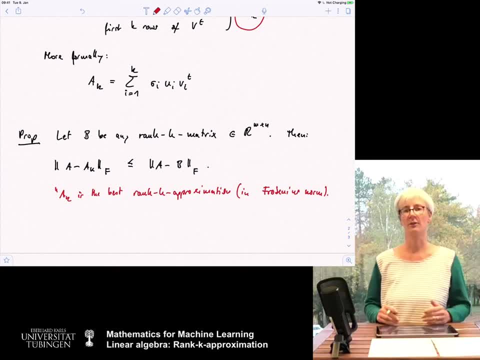 singular value decomposition and it's going to take too much time, but for me it is really important that you get the intuition. if we have a big matrix- m times n, a- and you want to approximate it with a matrix that's equally big but has a small rank, and this 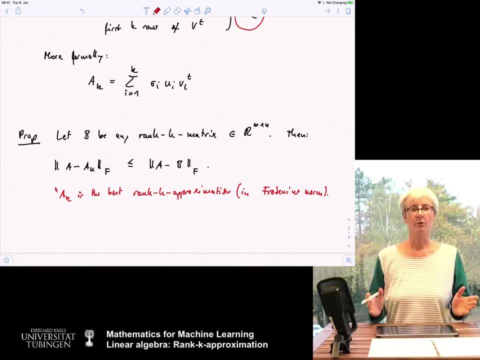 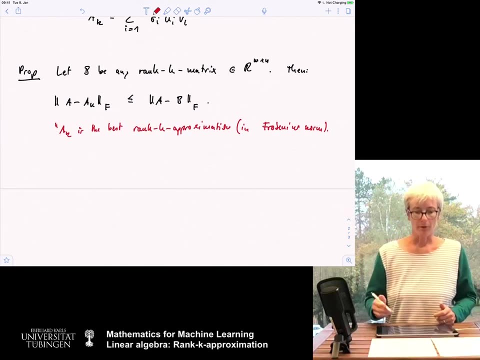 is something we often do in junior math machine learning- then the solution is going to be the SVD, and you can be sure that if you use the SVD, this is the best thing you can do, at least if you care about the Frobenius norm differences. Now, a similar theorem also holds for other 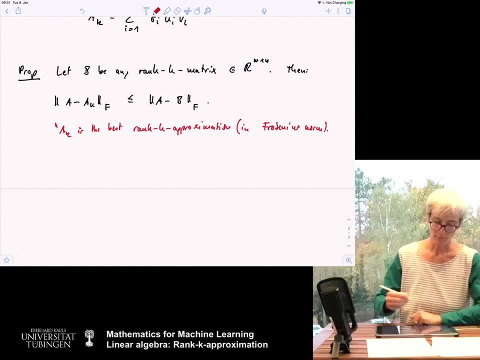 for the two norm, for the operator norm, And here it is sorry in black- for any matrix B of rank K and of course B it has the correct dimensions M times N. we have the B of rank K and of course B has the correct dimensions M times N. 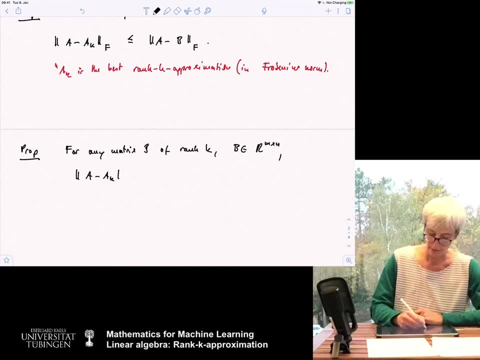 that if you compare now a and ak in the two norm, the operator norm, then again this is always a better than a minus b in the operator norm, maybe where i write it explicitly, where two denotes the operator norm, and so the intuition here is: ak is also the best approximation.